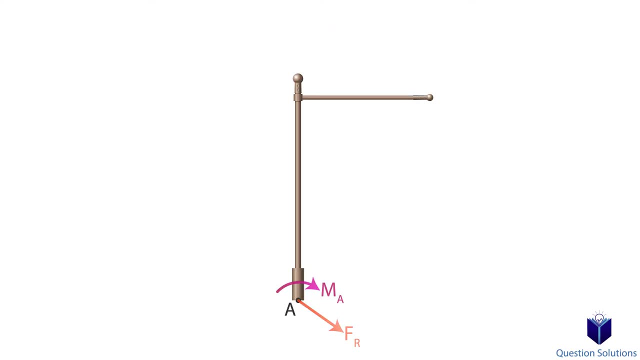 and a single couple moment that accounts for all the other forces. If we have an object in 3D space, the process is similar. We now express our forces in Cartesian form and add it up To find the moments. we use our trust equation and then, once we figure out the moments created by all the forces, 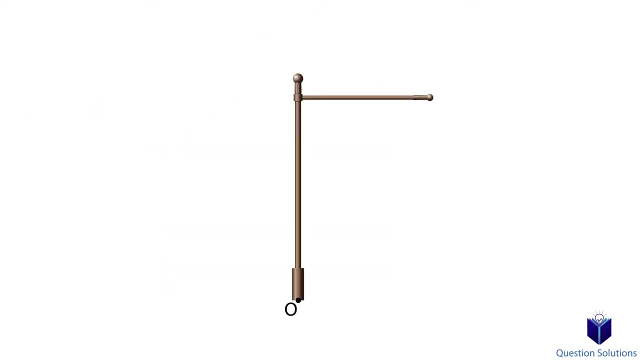 we can add it up. Now let's go back to our metal post. We can actually go one step further then show a couple moments that represent all the forces and moments affecting this post. Let's show a resultant and a couple moment. We don't even have to show a moment. Instead of showing: 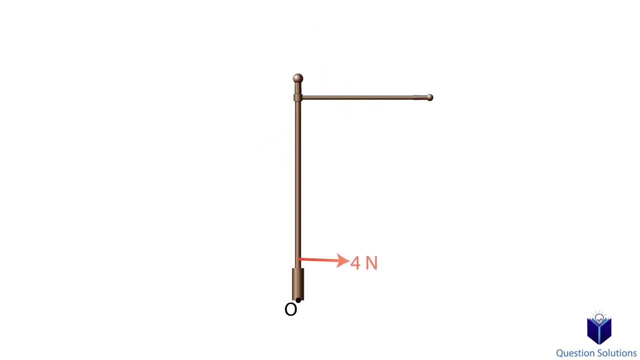 the couple moment. what if we can place our resultant force anywhere on the vertical post to account for the moment as well? In simple terms, we can show a single resultant force and place it somewhere on this vertical section, which will create the same couple moment we had before, Because, remember, it's force times, perpendicular distance. 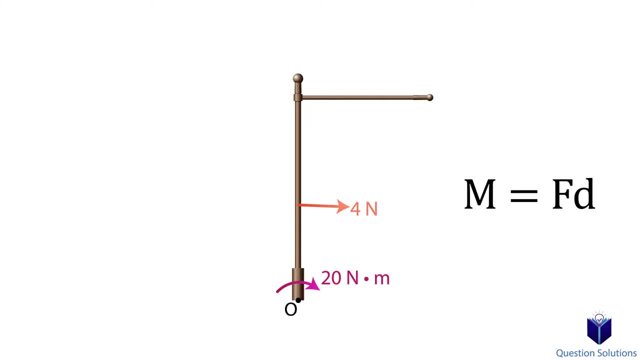 For example, if we had a couple moment of 20 Newton meters and our resultant force only had an x component of 4 Newtons, then all we need to do is place the resultant force 5 meters away from point O, and that would create a moment of 20 Newton meters. 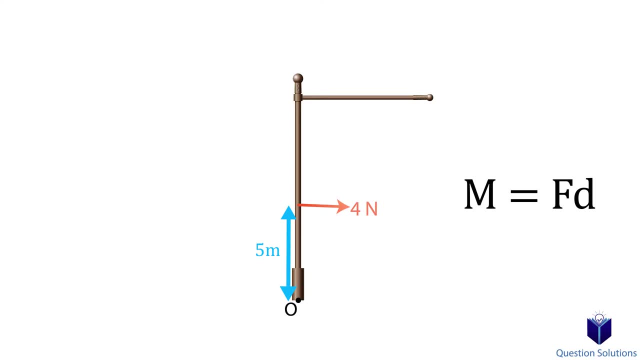 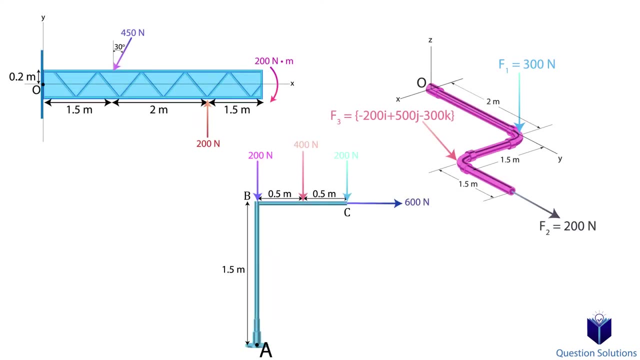 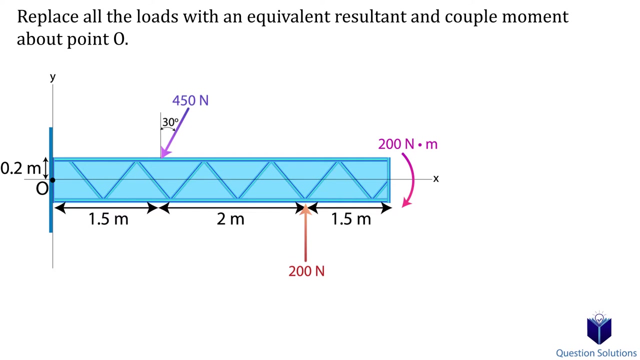 So now our resultant force accounts for the moment as well. We will do this in the very last example to see how it's done. Now we'll move on to some examples. Let's take a look at this problem, where we need to replace the forces and moments affecting the beam by an equivalent resultant. force and a couple moments. Let's take a look at this problem, where we need to replace the forces and moments affecting the beam by an equivalent resultant force and a couple moments. Let's take a look at this problem, where we need to replace the forces and moments affecting the beam by an equivalent resultant force and a couple moments at point O. 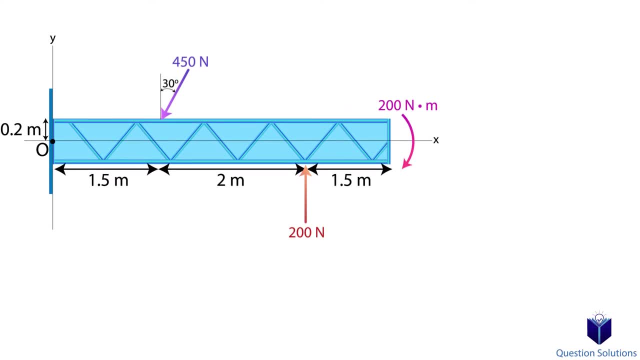 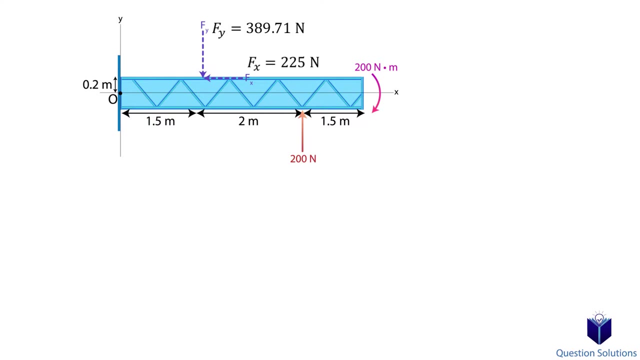 Let's start with the forces. The 450 Newton force can be broken into its x and y components. The 200 Newton force only has a y component, so we don't need to break it into separate components. Let's add up the forces. We will pick down and to the left to be positive. First the x components. 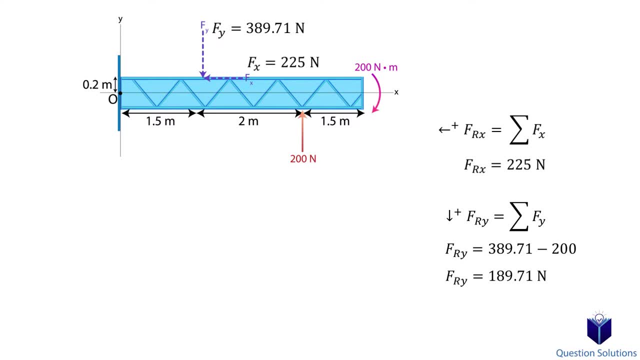 Now the y components. Note that since we picked down to be positive, the 200 Newton force, which is facing upwards, will be negative. Now we can find the resultant force by finding the magnitude. We also need an angle to show the direction of the resultant force. So let me draw out the components. Using tan, we can find: 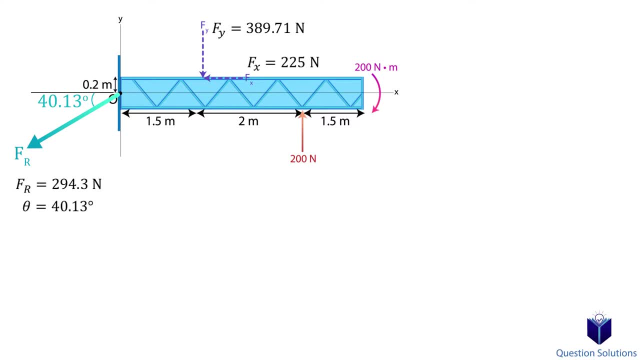 theta. That's the force taken care of. Let's move on to moments. Each component of the forces will create a moment. Let's look at the x components, which is only one force. The perpendicular distance is 0.2 meters, so we multiply the force by the distance. This would create a counterclockwise. 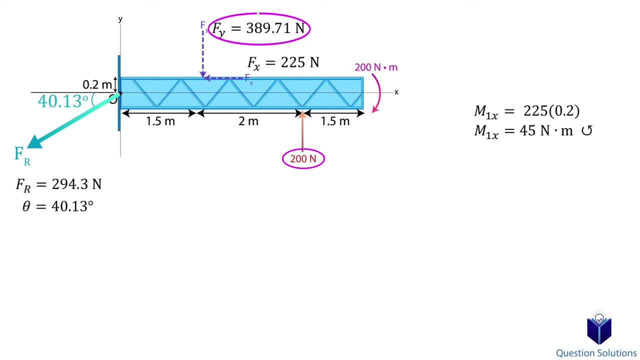 moment. Next we look at y components. We have two. Looking at the first force, we have a perpendicular distance of 1.5 meters. This would create a clockwise moment. Next we look at the 200 Newton force. The perpendicular distance is 3.5 meters. This would create a counterclockwise. 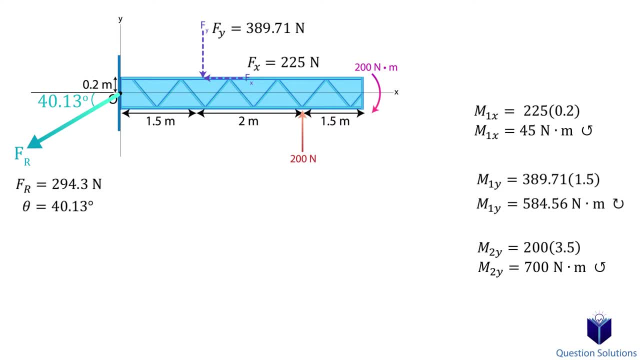 moment. Now there is one more moment that we need to keep in mind, which is already given to us. We will assume clockwise moments to be positive and add it up, So note that the y components are only one force. This would create a counterclockwise moment. 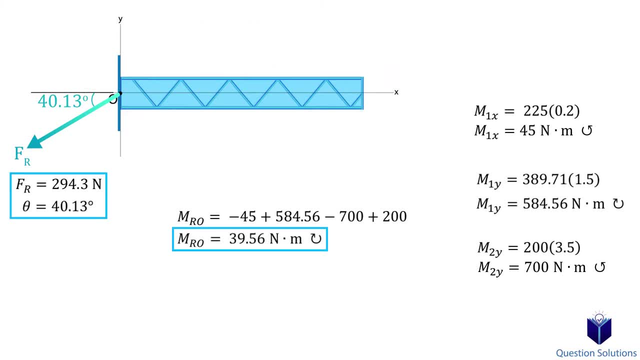 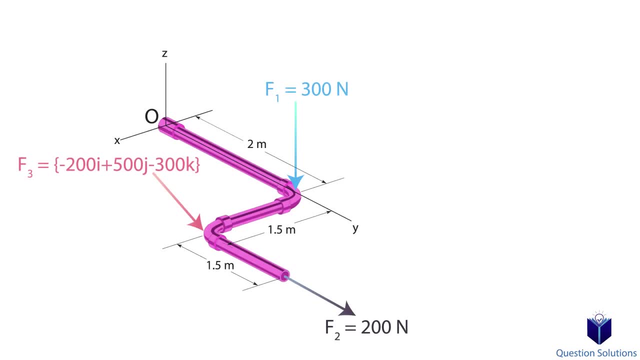 Note that all the counterclockwise moments will be negative, since we picked clockwise to be positive. Those are our answers. Let's take a look at a problem involving vector analysis. Same as before: we need to find an equivalent resultant force and a couple moment at point O. 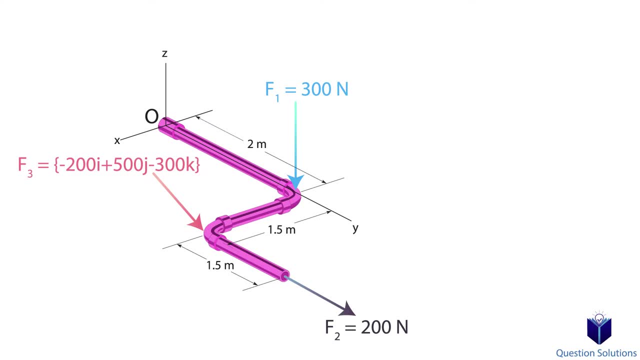 We will start with the forces first. Force F1 only has an z component, so we can write it like this in Cartesian form: Force F2 only has a y component, so we can write it like this: Force F3 is already given to us in Cartesian form. Now we can find the resultant force by: 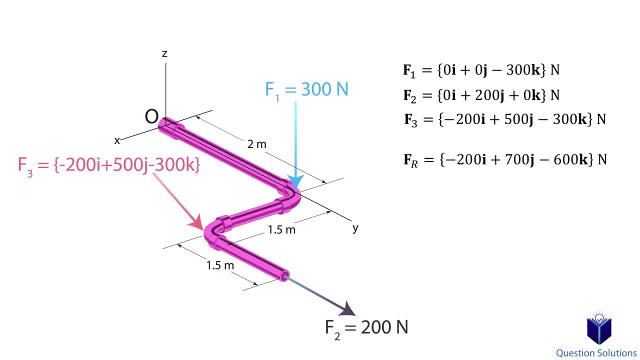 adding it all up. So remember, all we do is add the i components to i components, j components to j components and k components to k components. Next we look at the moments created above point O by each of the forces. So for force F1, we need a 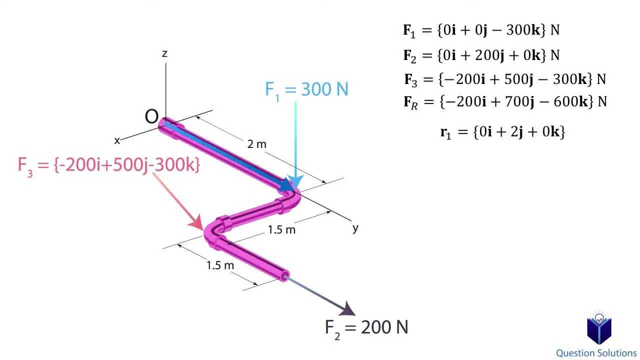 position vector from O to where force 1 is applied. For force F2, we need a position vector from O to where force 2 is applied. Lastly, for force F3, we need a position vector from point O to where force 3 is applied. Now we can find the moment by taking the cross product. Let's start with force. 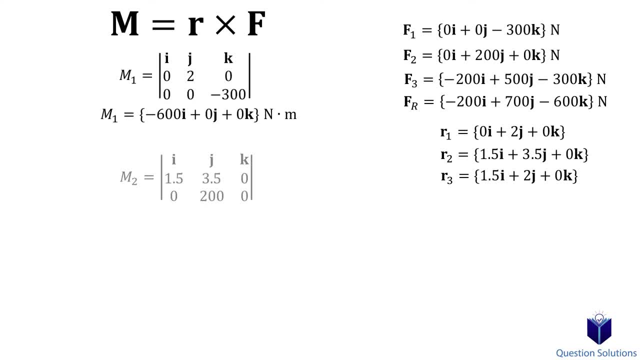 F1. Next force F2. And lastly, we have force F3.. Now to find the resultant moment, all we do is add it up, just like when we did the resultant force, and that's our answer In the previous two. 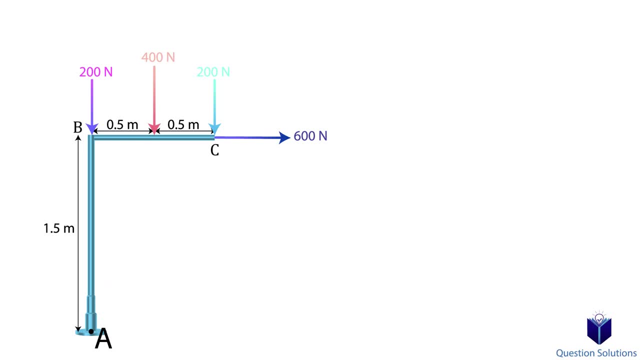 questions. we showed a resultant force and a moment about a specific point. Now we're going to go one step further and show the resultant force and place it at a location so that it accounts for the resultant moment as well. So let's take a look at this problem where we need. 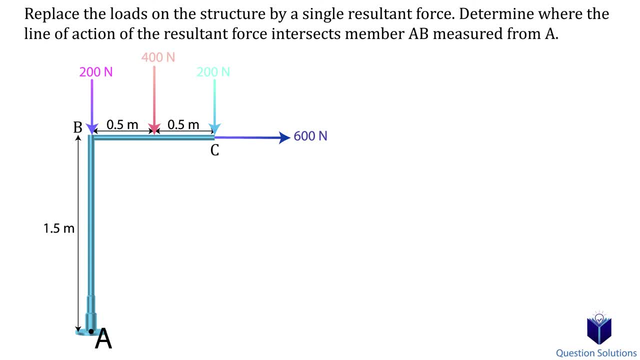 to represent the loading on the frame with a single resultant force. The method is similar to before. Let's start with the forces. First the x-axis forces. We will pick right to be positive and there's only one force. Next, y-axis forces. Using this, we can find the resultant force. 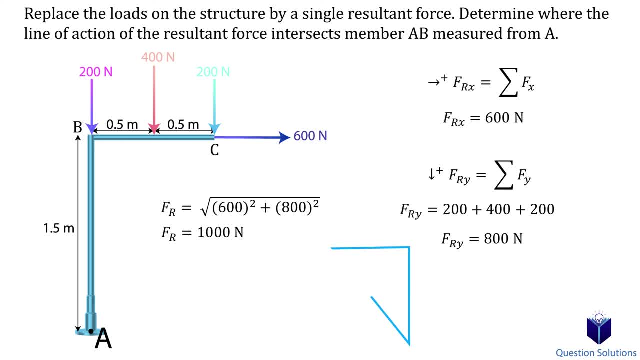 We also need an angle to show the direction. So let's draw the components Using tan inverse. we get the angle. Now we will set that aside and look at the moments created by the forces. Since the question is asking us to find the line of action from point A, we will calculate the 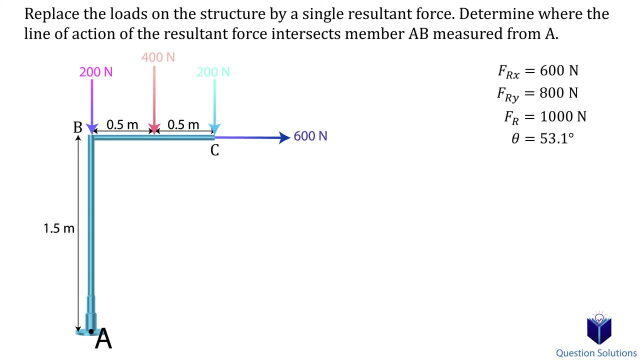 moments created. about point A: The first 200N force won't create a moment, since its line of action is 0.2N. The first 200N force won't create a moment, since its line of action is 0.2N. The 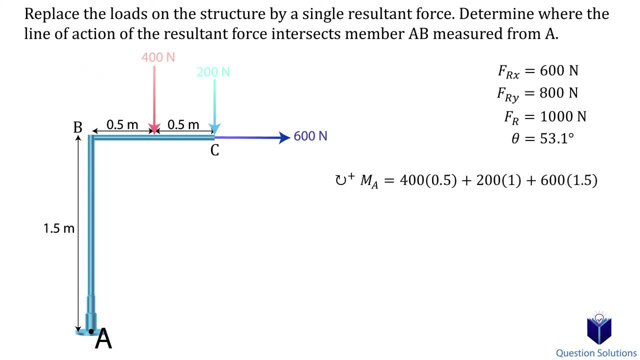 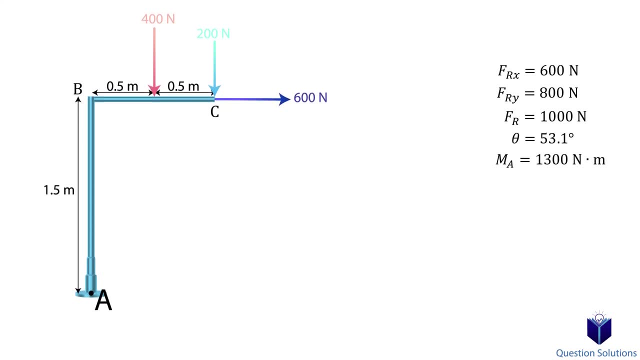 action intersects point A. The rest of the forces create moments. so let's figure it out: assuming clockwise moments to be positive, This tells us the resultant moment created by all the forces. Now, going back to the resultant force, we found we need to place it somewhere. 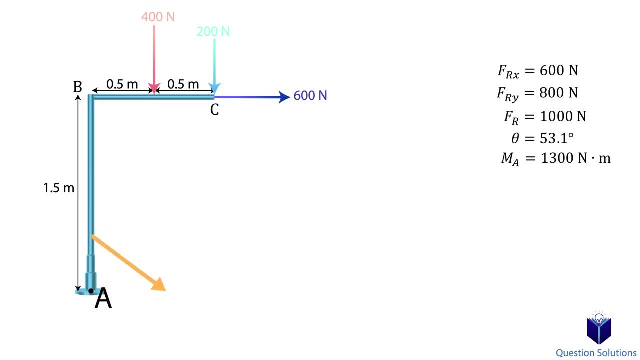 along this vertical bar so that we can account for the resultant moment. Since the y-component of our resultant force goes through the vertical line of member AB, we can ignore it. So where can we place our x-component to account for the moment? Well, let's assume that this. 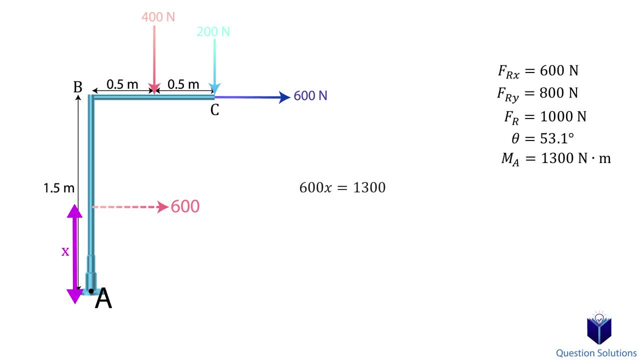 length is x, The moment created would be 600 times x, and we just need to equal that to the resultant moment. So what we're saying is that if we place our resultant force at this location, it will account for the resultant moment that's created as well. So in simple, 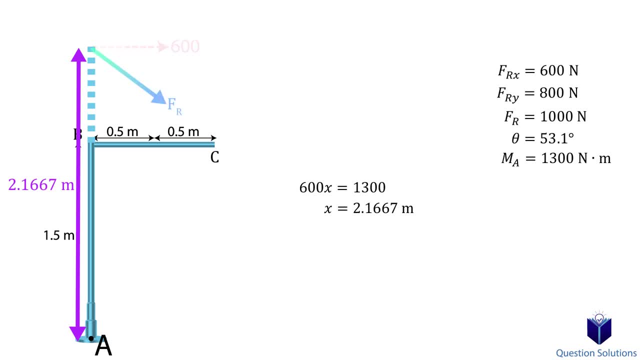 terms, we can replace all the forces that's on this beam with this single resultant force, and that's our answer. That should cover the types of problems you will face when it comes to simplification of forces and moments. I hope this video helped and thanks for watching. Best of luck with your studies.